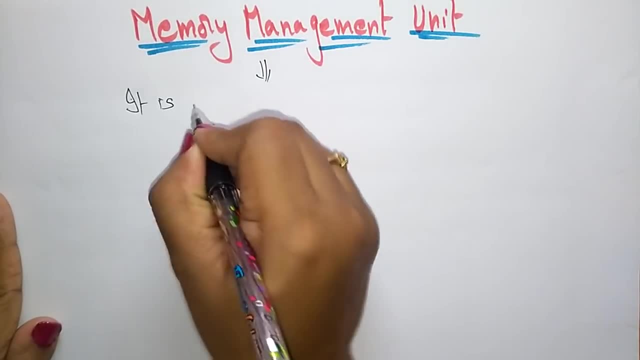 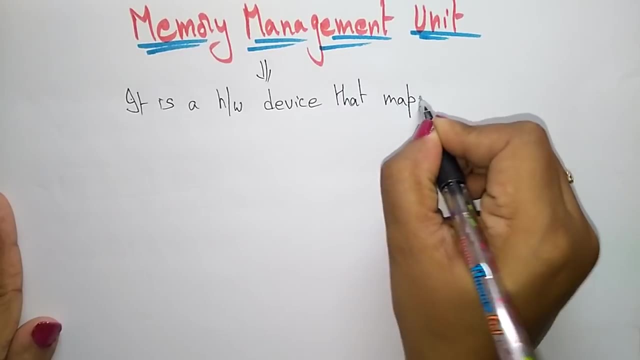 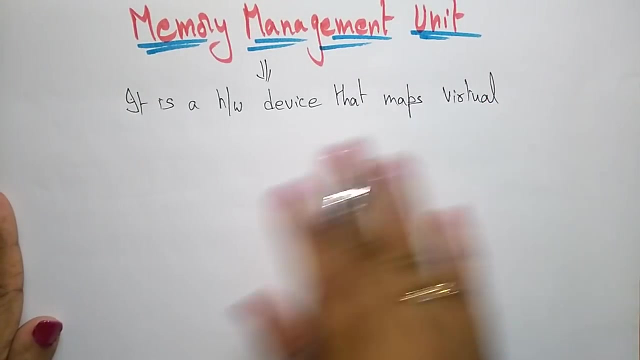 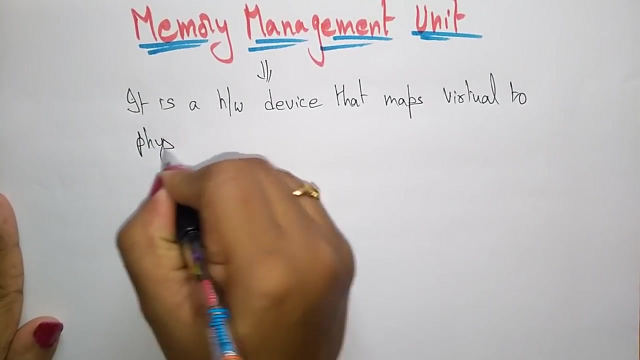 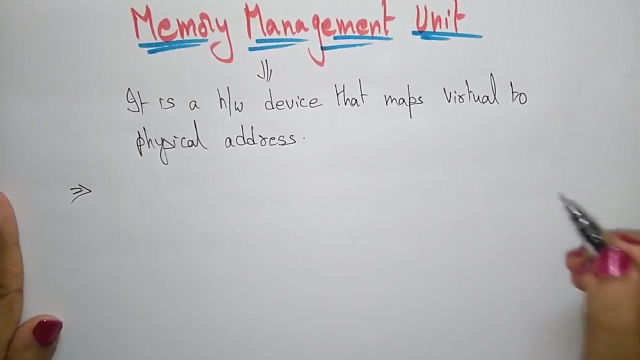 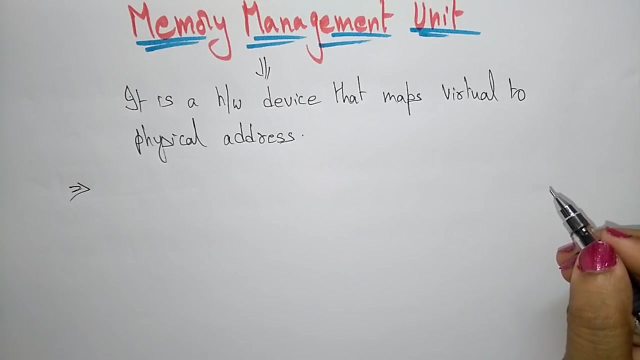 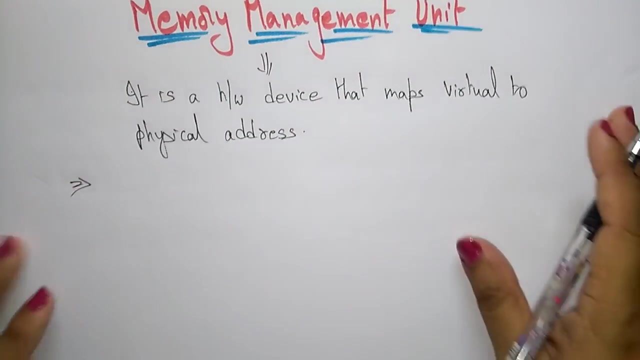 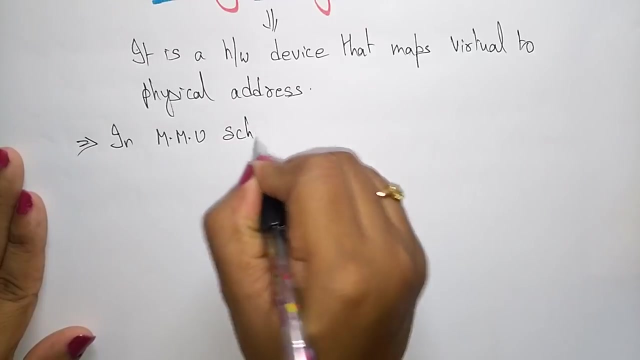 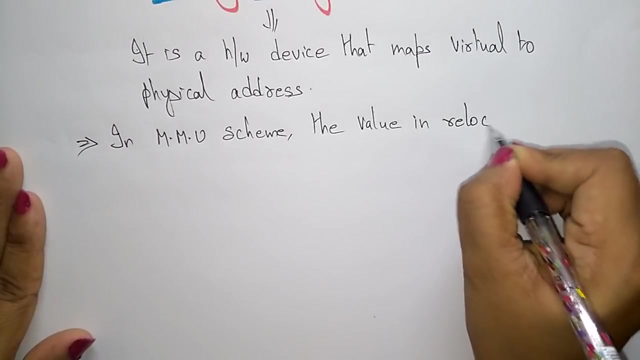 unit is a hardware device. It is a hardware device that maps virtual to. So virtual is nothing but logical. Don't be confused Logical and virtual, both are the same. So it is a hardware device that maps virtual to physical address. So in memory management unit scheme, the value is relocation. The value in relocation register is added to every address generated by the user process at the time it is sent to memory. First let me write the point, Then I'll explain with diagram. So in memory management unit scheme, the value, So it consisting of value, the value in relocation register. The memory management unit consisting of one relocation register is addressed- sorry- is added to every address. This point you have to remember. So the relocation register is added to every address generated by the user. So whatever the user process it's having at the time it is sent to memory. 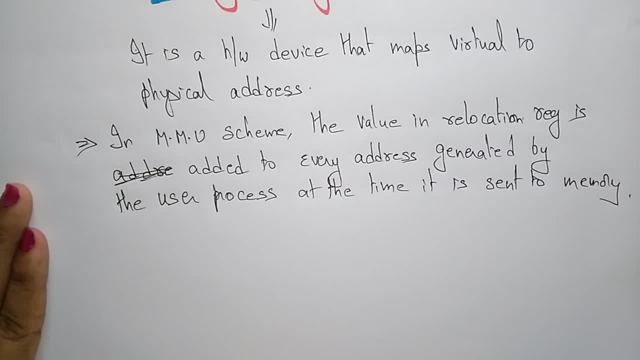 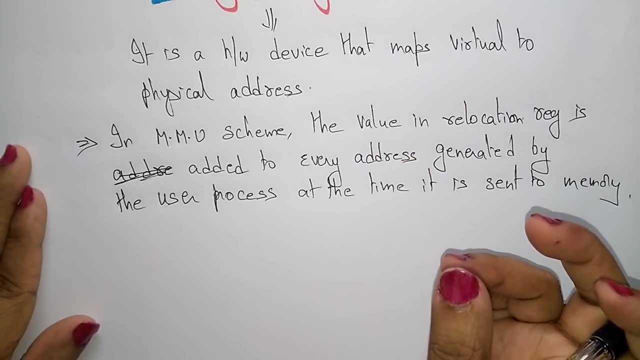 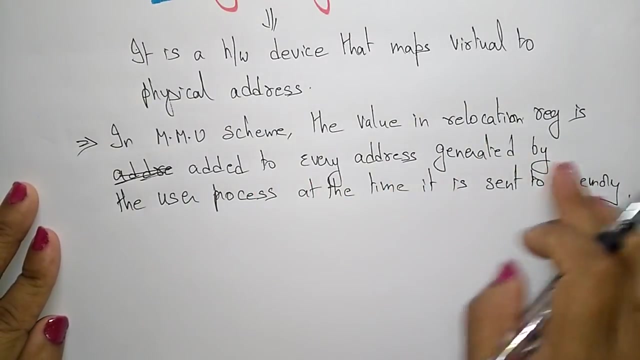 So here what it's saying in memory management unit scheme. it consisting of some: the value that, whatever the value that is present in the memory management unit that is real in relocation register is added to every address generated by the user process at the time it is sent to memory. memory is a physical memory i am talking about here. 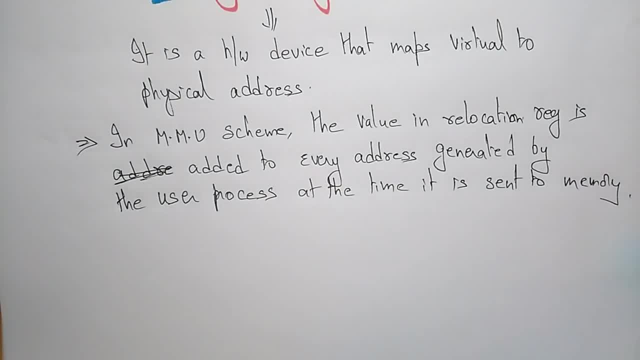 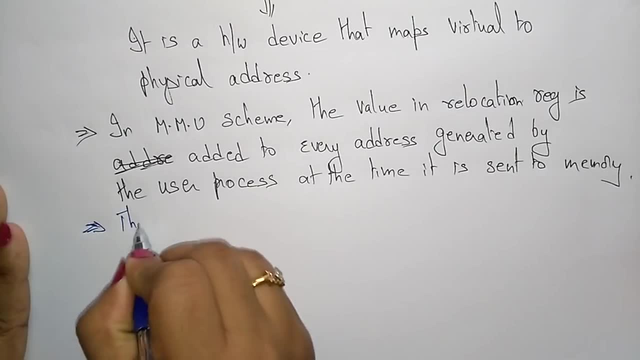 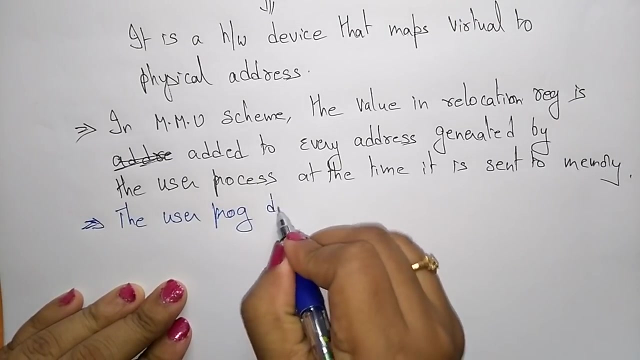 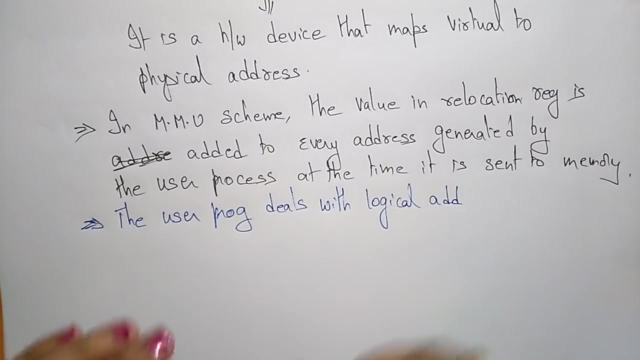 the user program deals with logical address. it never sees a real physical address. so, whatever it is consisting of the user program- this point you have to be remember- the user program, whatever we have written, so that user program always deals with logical address, because the user doesn't know whatever he is returning. uh, that come, actually the whatever. 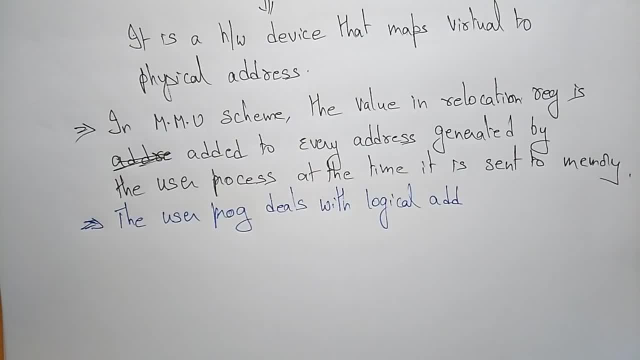 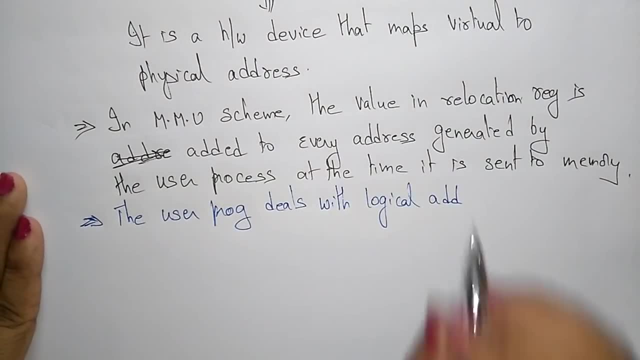 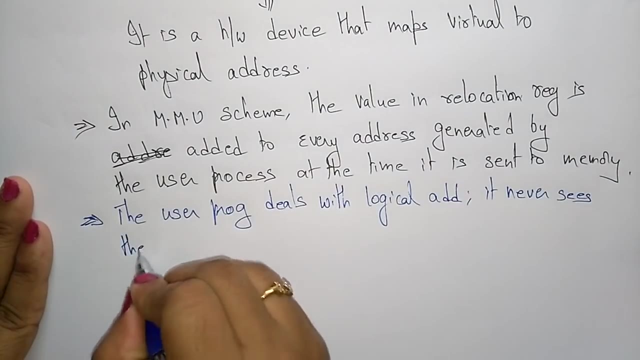 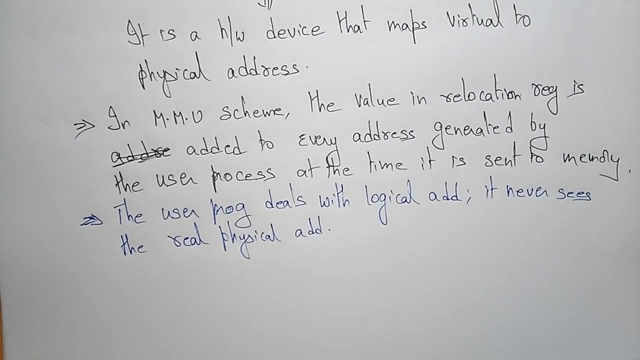 the program that we are writing, that the program size is, uh, larger than the physical memory. that is a memory, uh memory unit. so the user program always deals with the logical address. it never sees the real physical address. so we always use it to write lot, of, lot of program steps, or, uh, we are always executing a large amount. 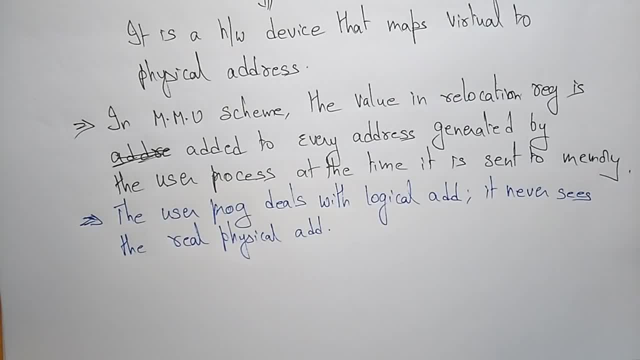 of data in the system. but whatever you are returning uh, that is more than larger than the physical memory, whatever you are having in the system. so this uh program first, the cpu deals with the logical address only the uh wanted information, so that will be stored in the physical. 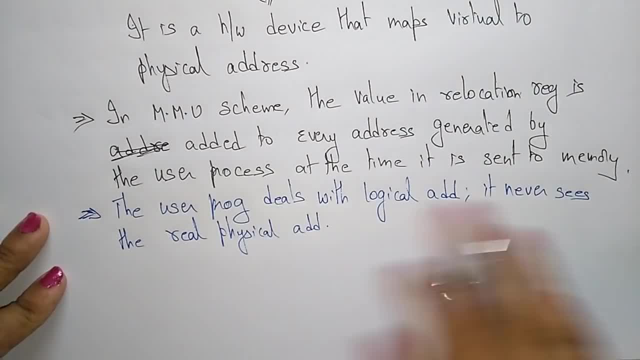 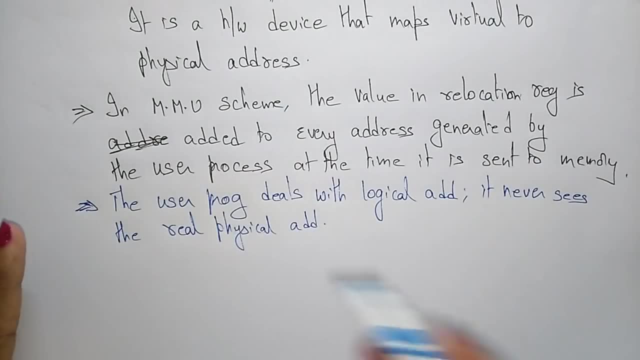 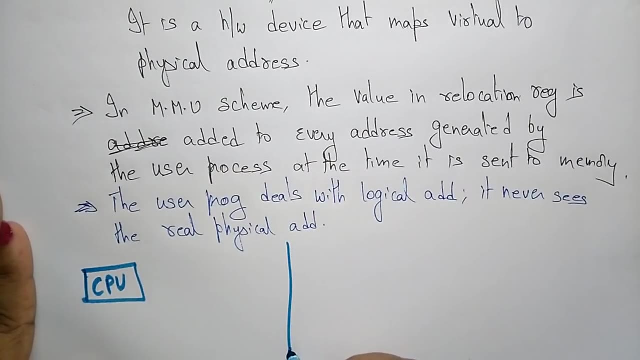 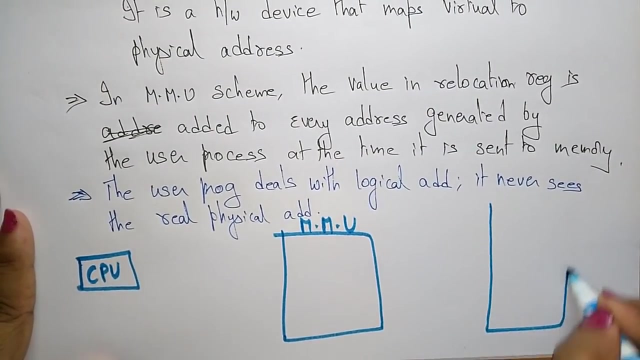 memory. so the user program always deals with the logical letter. it never sees the real physical address. so let me explain this: what this memory management unit scheme suppose here? this is a cpu, okay, and here you are having the memory management unit and this is. let take, this is the physical address. 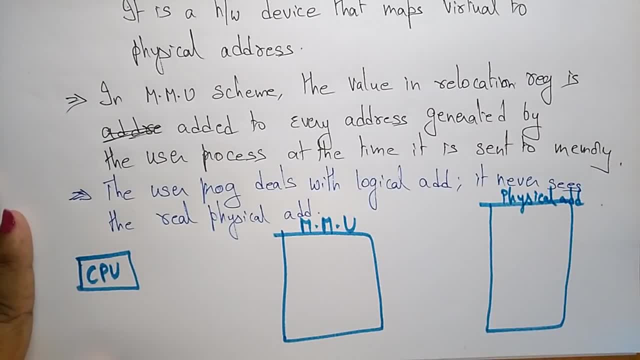 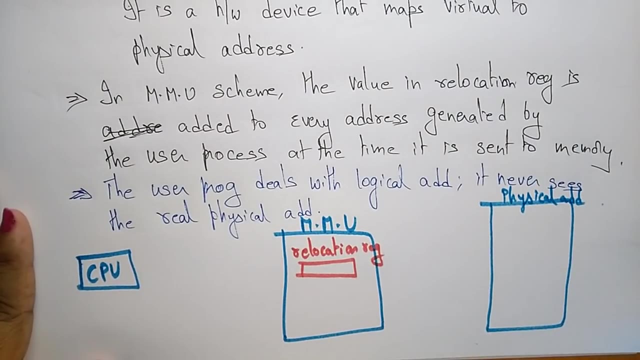 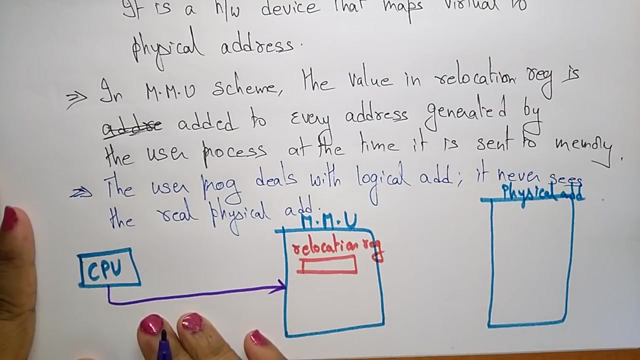 or you call it as a memory unit. okay, so here in memory management you need some relocation register. will be there, so this is a relocation register. so the cpu wants to sense the data, so it is sending some logical address. let us take this logical address is 346.. the address of that data, uh, whole. 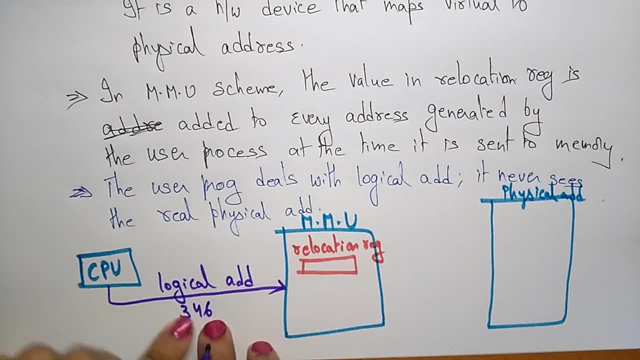 that logical address is 346, so that 346 will send to that wants to sense, to the physical memory. so this logical address is added to this relocation register, so the relocation register consisting of 14 000. let us take so what you are saying in memory management. 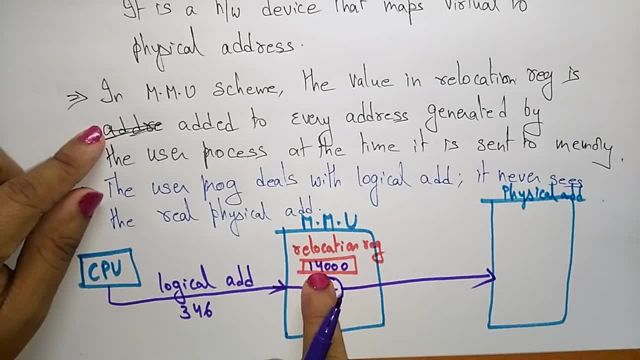 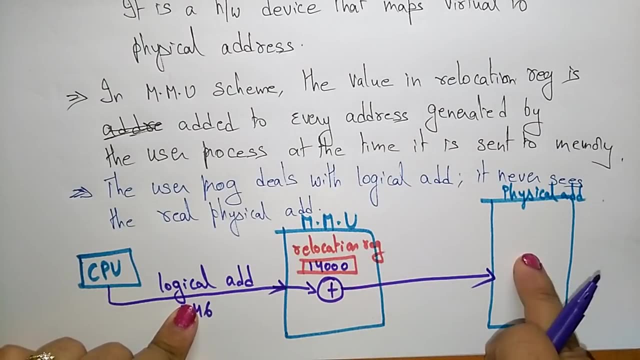 unit schema. the value in relocation register is added to every address generated by the user process. So this is a user program. The user process is generating one address, So that address will be added to the relocation register at the time it is sent to memory. So at the time of sending to the memory the logical address will be added to the relocation register. 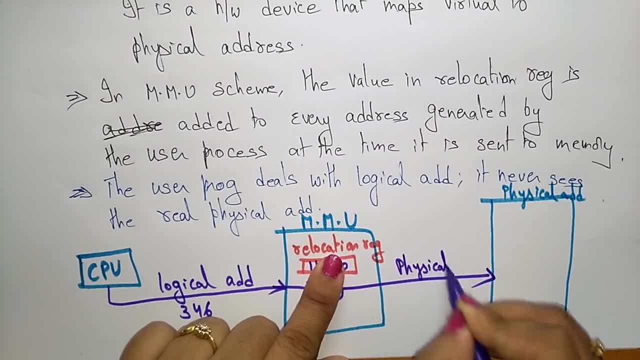 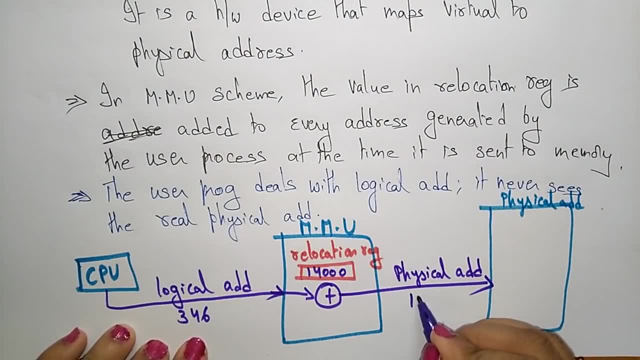 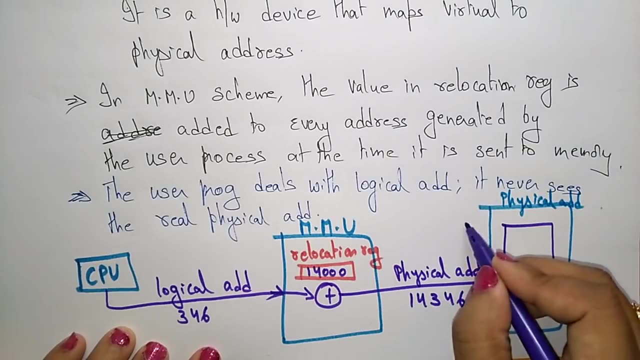 So now what is the physical address? The physical address is the user process address, that is a logical address plus relocation register, So total 14346.. So which is present in this physical memory? So here this is address. starting will be the 14000. So it will be stored the data up to 14346.. So this is relocated code.